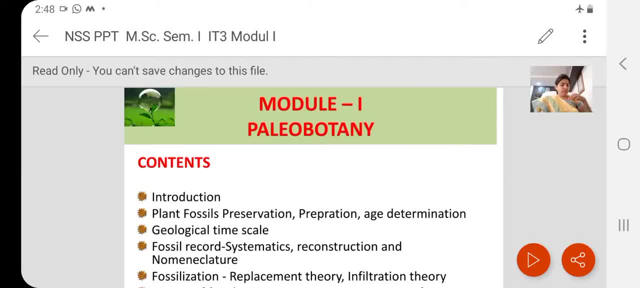 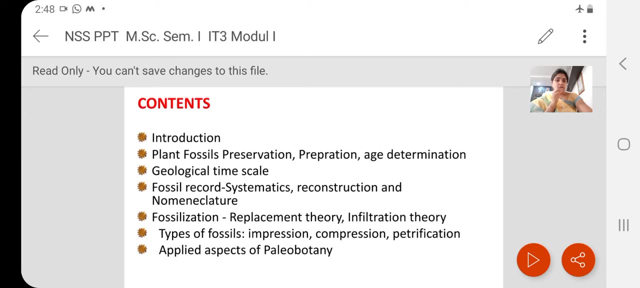 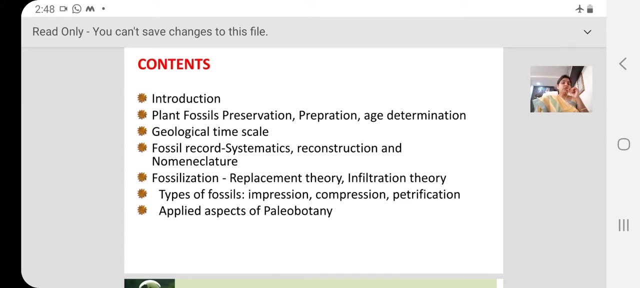 Hello students, I am Dr Naina Shilbharte from Vidyavikas College, Samudrapur. Today we will discuss about the different aspects of paleobotany. In this lecture we have discussed these points. That is the introduction of paleobotany. Then in this lecture we have detailed study on geological time scales. 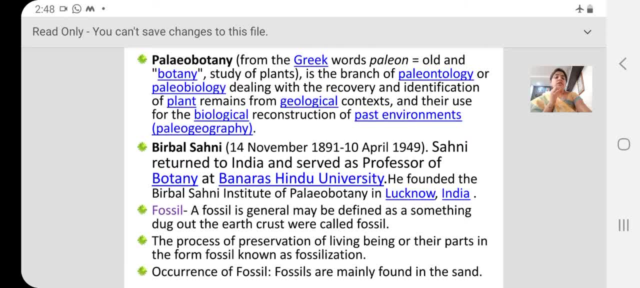 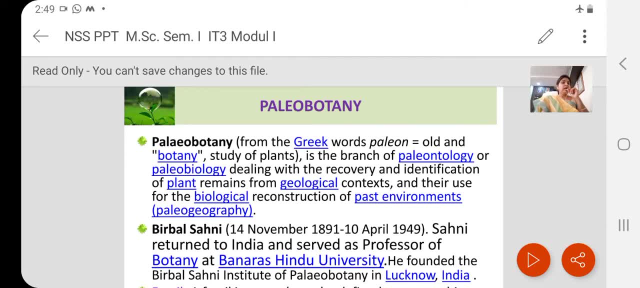 Okay, Now I am start. what is the paleobotany? Paleobotany, from the Greek word paleon means the old and botany. it is the study of plant. It is the branch of paleontology or paleobiology dealing with the recovery and identification of plant remains from geological contents and their use for biological reconstruction of past environment. 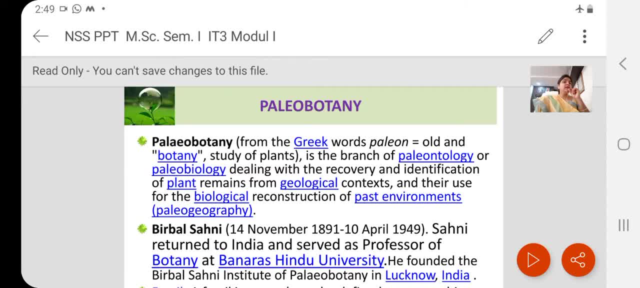 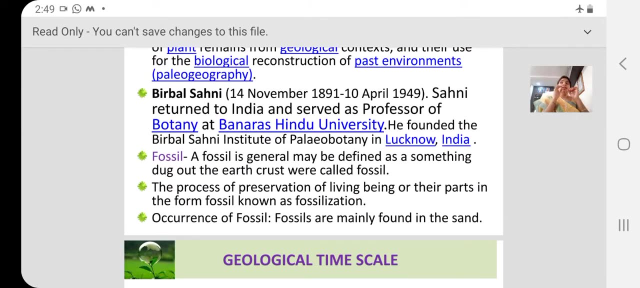 Okay, Paleobotany is nothing but the study of plant. Okay, The study of fossil is known as the paleobotany And the. and what is the fossil Fossil? something dug out, the earth crust, Something dug out the earth crust were called fossil, And the study of fossil is known as the paleonopalogy. Okay, 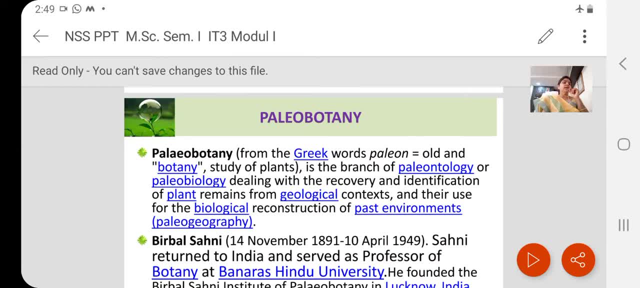 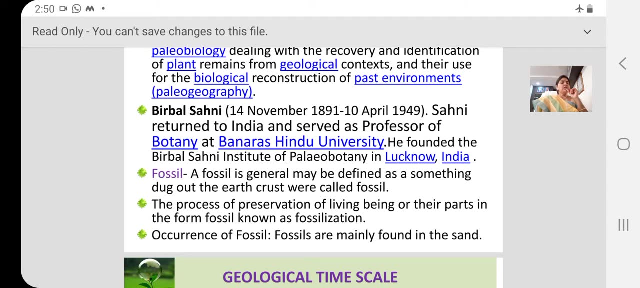 Paleobotany, or paleobotany Birbal Sahani returned to India and served as a professor of botany at Banaras Hindu University, And he founded Birbal Sahani Institute of Paleobotany in Lucknow, India, And in this institute store number of fossils or other geological evidences. Okay, 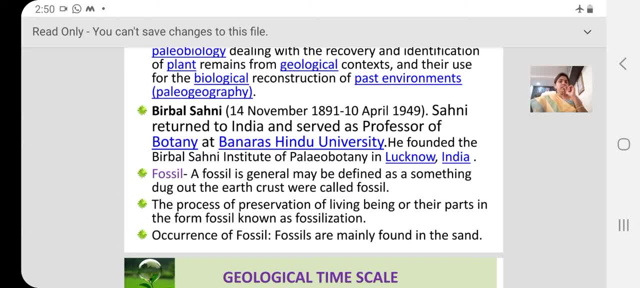 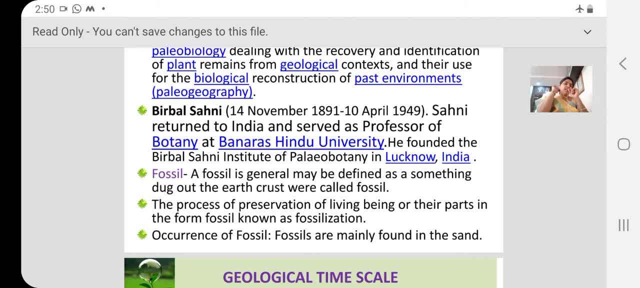 The study of fossil is known as the paleobotany, And in this institute store number of fossils or other geological evidences. Okay, something dug out. the earth crust were called fossil. the process of preservation of living being or their parts in the form of fossil, known as the fossilization. 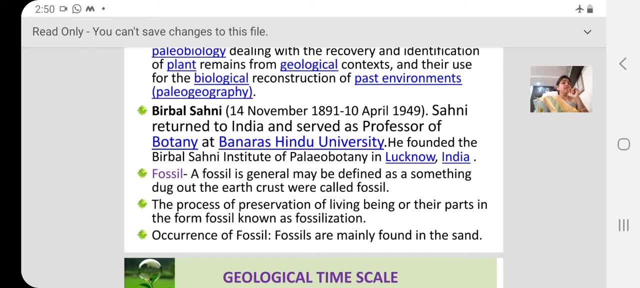 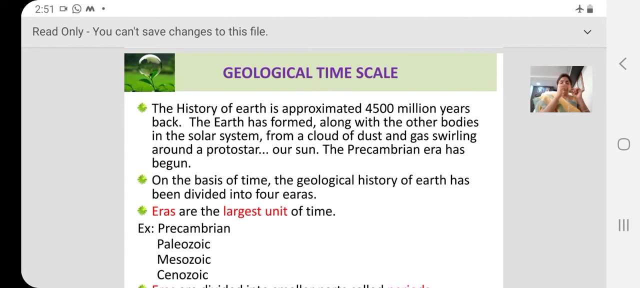 the process of preservation of living beings, okay, or their parts in the form of fossil, known as the fossilization and occurrence of fossil. Singha and and geological timescale history of earth approximately 4500 million years back. the earth has formed 4500 million years back. 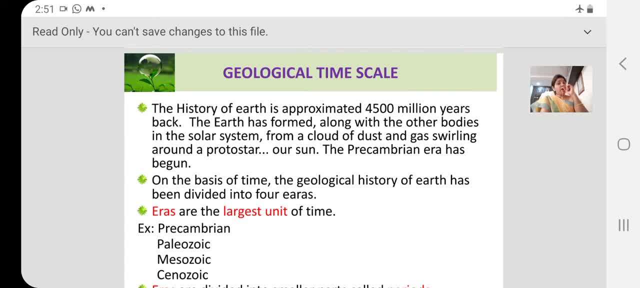 4500 million years back. the. the earth has formed millions years. earth formed, along with other bodies in the solar system, From clouds of dust and gases gas swirling around a protostar. the pre-cambium era has begun. You can see the video lectures on how the earth formed online. 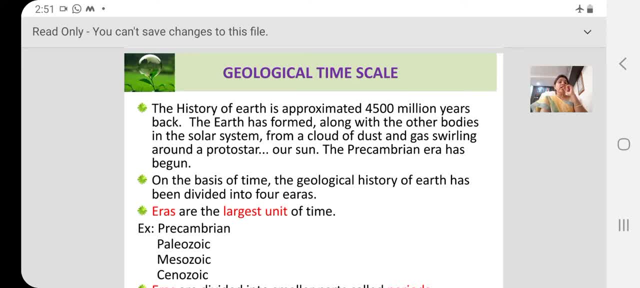 On the basis of time, the geological history of the earth has been divided into four eras. Geological history has not been divided into four eras. It has been divided into number of periods, and number of periods has been divided into epochs. Like we say year: how many months are there in a year? 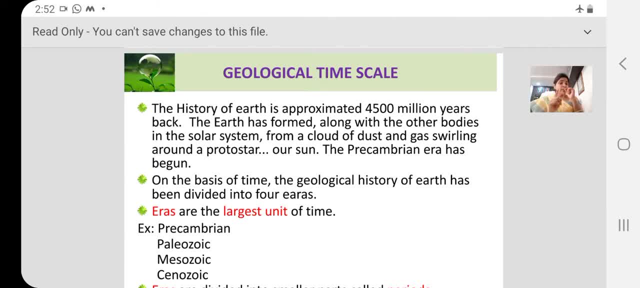 Twelve, Twelve months, How many weeks are there in a month? Four, How many days are there in a week? Seven? Similarly, the entire history of the earth, whatever years have passed since its formation, has been divided into number of eras. 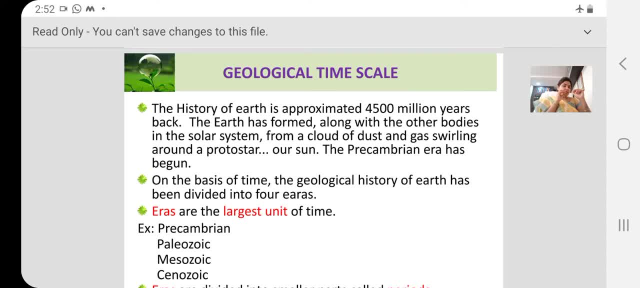 It has been divided in to four eras: Precambrium, Paleozoic, Cenozoic. Like we have divided the year into twelve months. Next there are the periods of the pre-cambrian era Paleozoic. How many years have they been found? 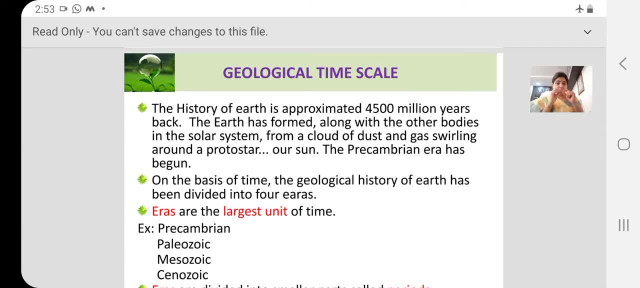 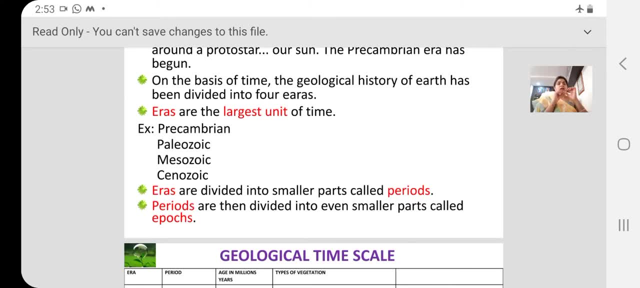 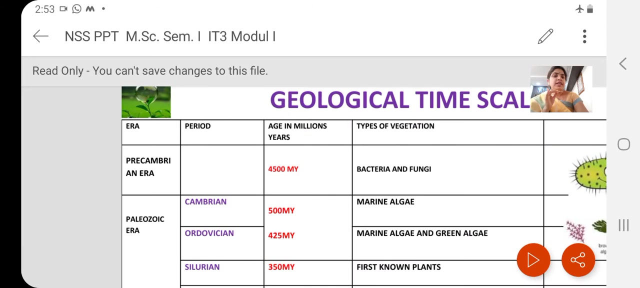 How many years have they been found? How many years have they been found? the sapon month: la puna divide Kerala, heavy comedy. okay, that's it. the periods are then divided into even smaller parts called the epics. okay, the atabag open geological timescale. okay, at the ha geological timescale. but I 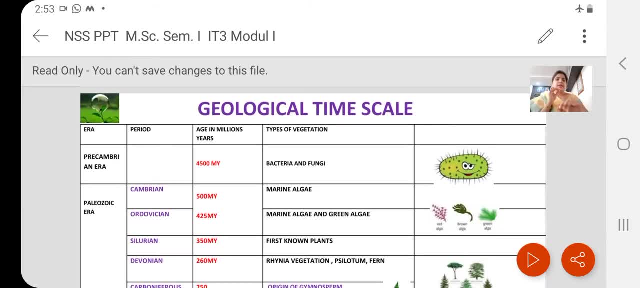 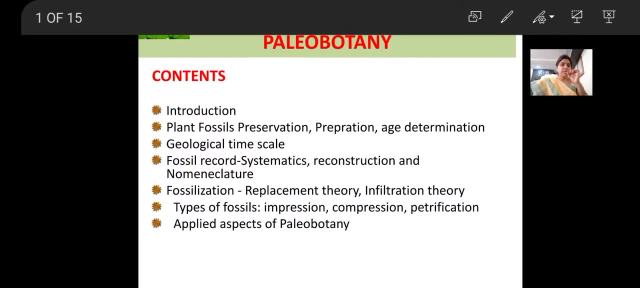 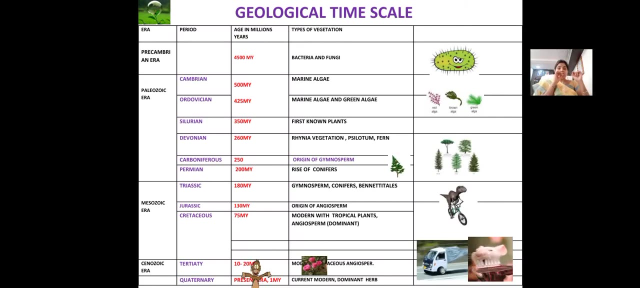 it's a Sala that, but it's a bugger at Amala. he's like choker, talented as the better ones. I okay current bug at Amish last night show. well, I porno slides for hell. I mean at the heck cuz, sir, inventions are a lead pilot, malati. 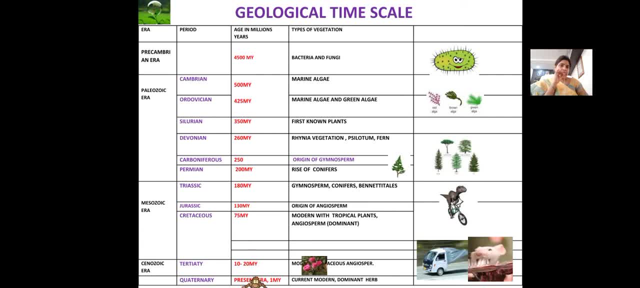 green, this, that algae. Bertie Tannan, ter chote, chote plant list at a hit up and bug week record. a cook lab pirates love a girl, a little car, so they for like. plan this at the head and third corn bearing, plan this at the hedges. a gymnast panic plant, a one so and so talent. the dinosaurs, a chitra. 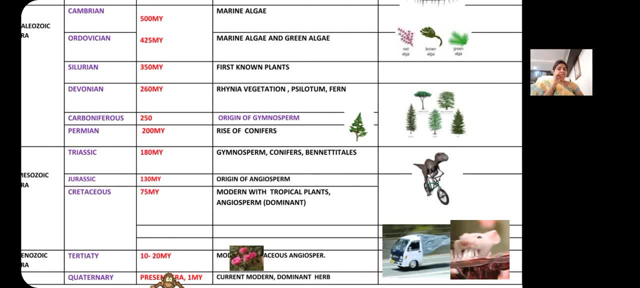 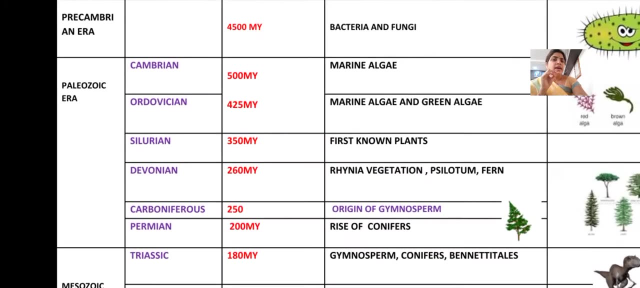 guard Leila HM a day and it then enter kakar Leila hey. yeah, that's a, you can have like them fast. okay, they cut Leila than me. that bug open plants, but it's up little actually detail mother tap and bagu plants of Kasuga, he's a Leila, hey. 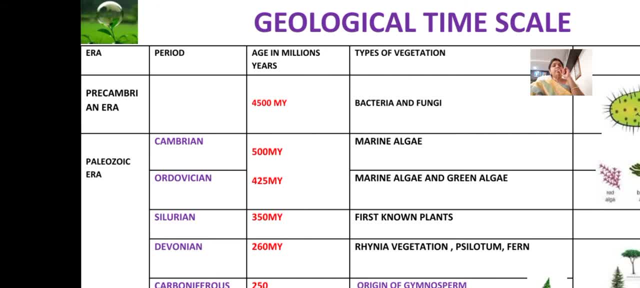 okay, then bugger, chop. ila hearing hit the peak. I am D&ER要, Dominic, that you might kill a very night the Camden Iraq. so hair could be starts. Allah, four thousand five hundred millions years ago. okay, Daewha Chiwood, urth Kaiti bacteria and f frågor bacteria. oмерa veterans regardless. 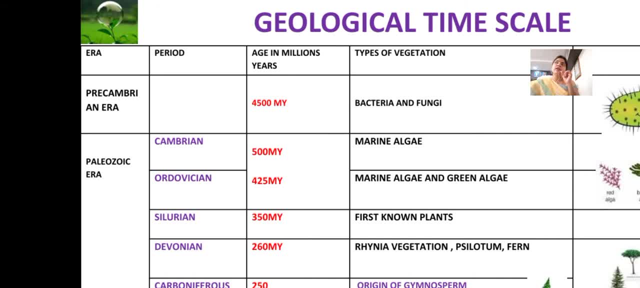 to the chile? hit okay, and fungi, fungi, bacteria might. and that's how, to the years? fungus, jr Dursi, he. pre-cambrian era, Madhavi volatility, okay. then enter the second era: hit okay, hey. paleozoic era: yeah, paleozoic idel a jayah, it would not. 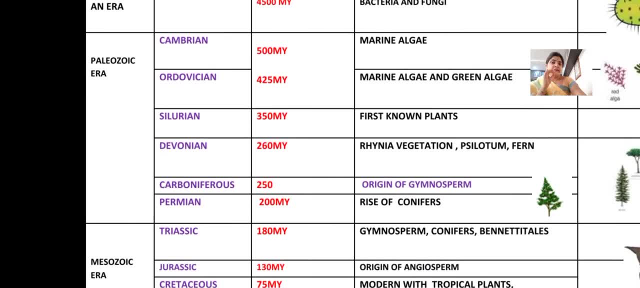 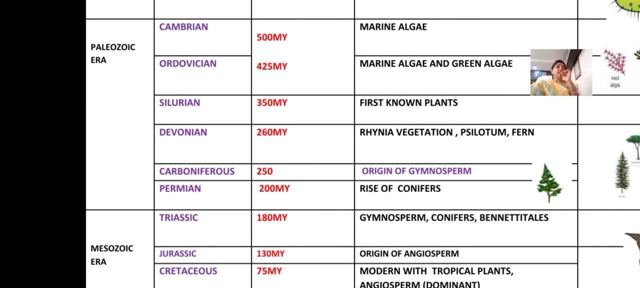 fire periods, mother divide, kill a gorilla. six periods man. okay, that's a pile up in a heck cambrian. second, a hey, or do we see? and third, a silurian. for the head, the onion fifth, a hey, carboniferous, and for the six a hey. 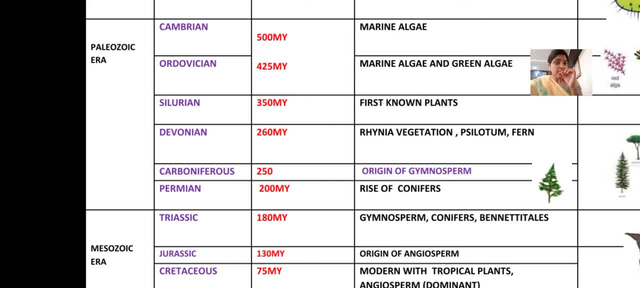 Permian. okay, hey to Malawi was the character. hey, Karen, yeah, periods, were these? kavi, Charlie, let Baroque questions which are Lillie. I took job John line exam on our head that a mother put no object to a hit paleozoic change. a period said could let six periods mother divide, kill a. 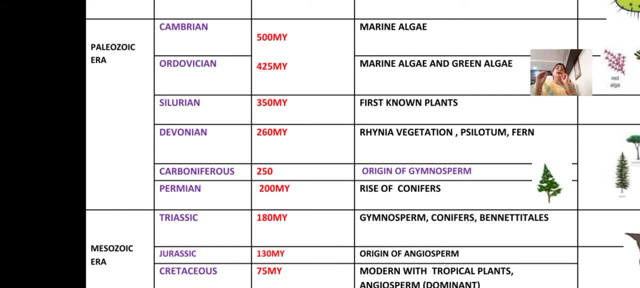 cambrian or do we see and silurian the onion carboniferous Permian other the question which are that? could lapidary de Madeira lucky involves a lady? a could lapidary de Madeira plants evolves a little? a could lapidary de Madeira. gymnos perms a original. okay, the to make a single gymnos firm originated in carboniferous period. okay, in 250 millions years ago. okay, I cannot the pile up a red book. cambrian period, cambrian period- kitty, who the years five hundred millions years ago? 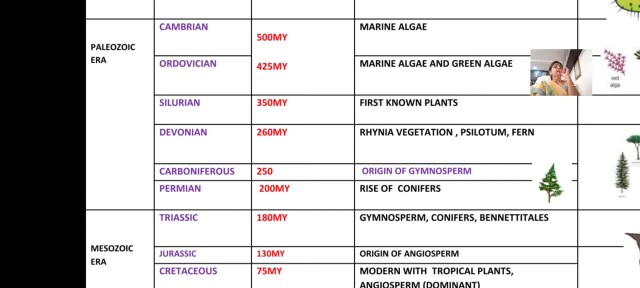 cahoot, a cambrian period of the Teva kai develops a lily, a marine algae. G Samudra tear again, oh, the sir saryasam G LGA the Samudra made a go to that al-ghad, al-ghad, al-ghad. Mariah Nalgi T Kadhi Houthi, cambrian period- mother. 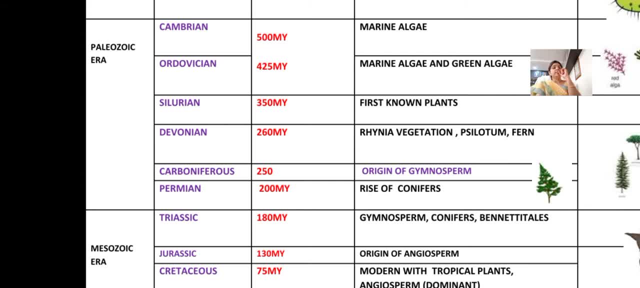 tanenter or do we see, and so period- I hate that I'm a day took a discharge, a lot four, and then 25 millions years ago and, yeah, period made a character: Mariah Nalgi and green. so combination of the 네- podal key, and green algae tannant, the celerian period. 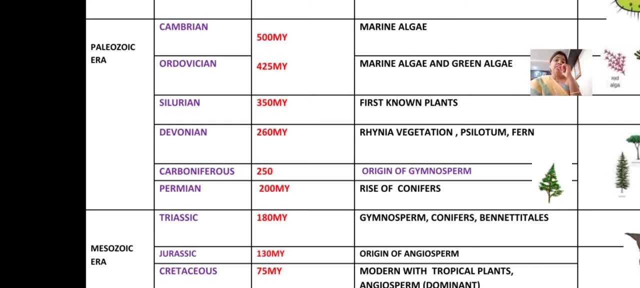 ahead. yes, a lurian period, Madhaka Oto, 350 millions years ago, a period Dutta and in touch with a force known plant, but he'll a plant: mela, okay, just a mini Verti. Mati Modeh, Appella Pilemere. okay, turn on. third EON, Ian period, the 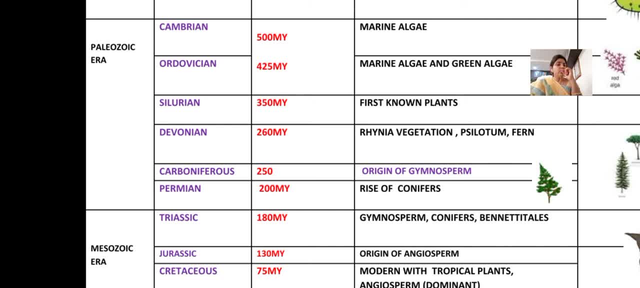 start Sarah, 260 millions years ago, okay, yeah, made a cooked hip plans, the ever are a rainy ahead vegetation, then the siloed term, phone, etc. then the next period. so I hate. oh hey, carboniferous spirit, how about a 250 million years ago? and he appeared, made a cave, all the origin of gymnosperm. okay, then enter. 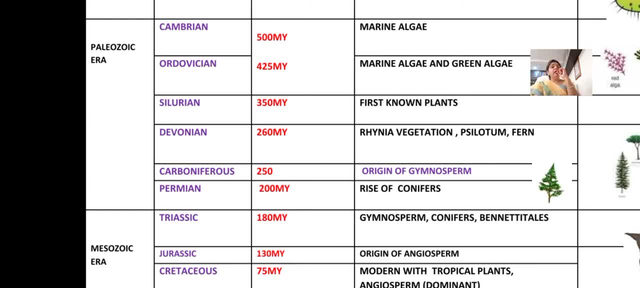 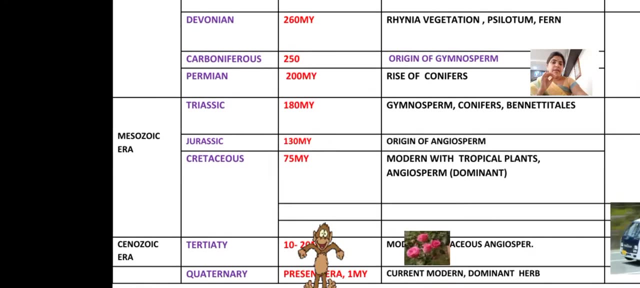 Permian period of that 200 million years ago. and he is a medic. I produce, can Halle, conifers, cone bearing plant gymnosperms. as a part, I hate cone bearing plant. that is the rise of conifers. okay, then entered he. casual failures, oikira up and at the third era, baguette lahe. mezozoic era. yeah, mezozoic. 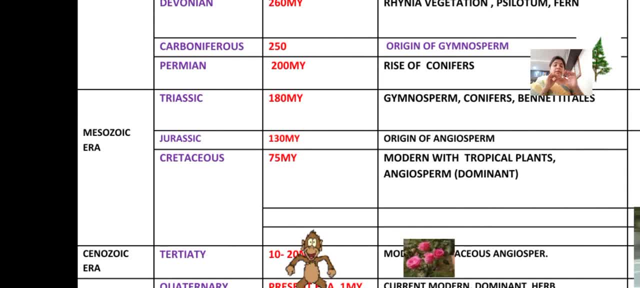 era modica baguette, sapla. la number of period, three periods where they had divide Salela. hey, try a sick period 180 million years ago. it's a medic I can develop. so they gymnosperm conifers and many titans. okay, and just come to Jay and sister with a benita, tells happen, it is evolved. 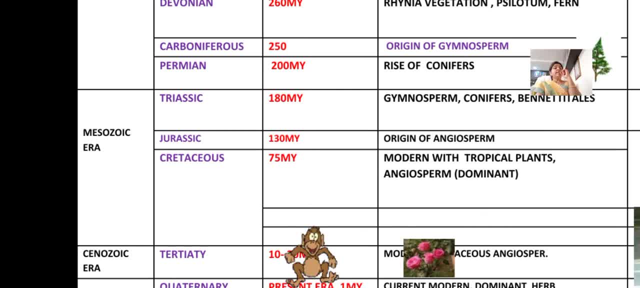 Salela hit, that's pretty mother. tell it the Jurassic period mother, 130 millions years ago. I produce a legim. no sperm, gymnosperm evolved in Jurassic period. he looks at the way. second equal, I origin Salela. hey, okay. Cretaceous mother, I produce a little a 75 million years ago. more done with tropical plants. 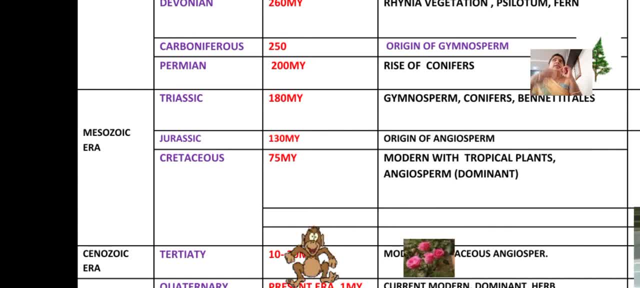 and and just pump. dominant Jan just playing a parameter. top Lilla, it's a somebody. word a hey, okay, Manjee Farah Indica, that is the mango than enter. word a heaven da, okay, when the entry that heck adept origin, it's a laylach. it hurt a serious period, but they me just wake. erasure okay, tan, until. 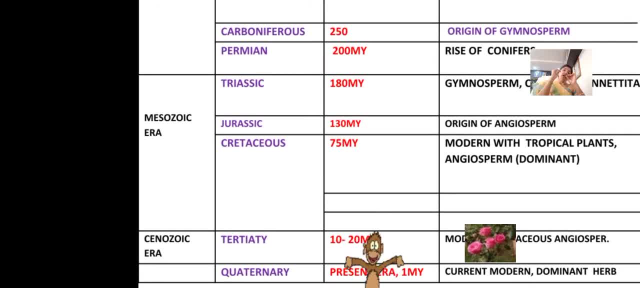 Cino's away. Mira, Jo hay, tell up una divide Kelly ahead, tertiary period. and 乙 Rt parrots mother ticket. see notice, like a descent era ha solaceata 10 to 20 million years ago, tertiary period. ota, it's a mother and juice pump mono del. 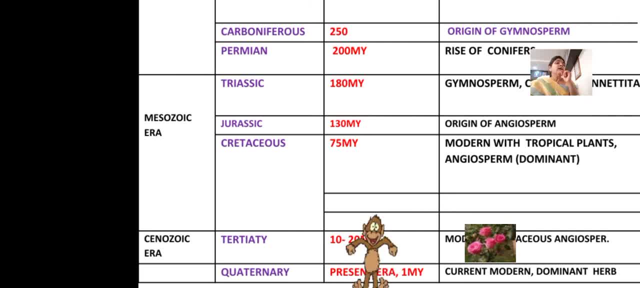 free monaceous and juice pumps? Jahe, they would they. they are monocotyledons and dicotyledons. so, Malama, it is okay, case our cages. how do they take a monocotyledon as plants and lilia? hey, okay, Nishigandha. he who are he chavar? hey? 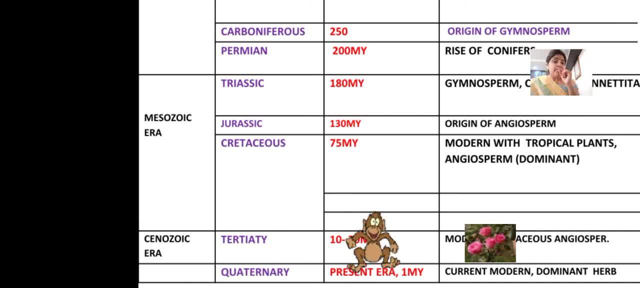 Paziri, hey, okay, he came monocotyledon as plants. I hate it. tertiary parade mother and a cotton. quaternary parade mother: the sub present era. so hey, 1 million years ago, current modern dominant herb: gymnos, pomada, diversity, pahala, mate and juice, permac plant, jahit, advanced plant, the 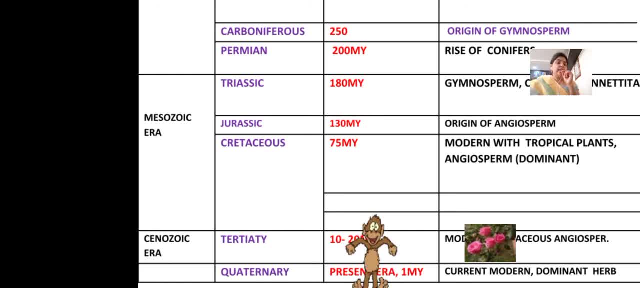 beer Silla's a Leila and juice permac plant- I'm a the way vegan term to mr Leila. this a herbaceous plant that sure by hip freeze ahead. okay, there, dominant herb jahit the appellate pahala. merrily ahead, yeah, cotton. Marie. 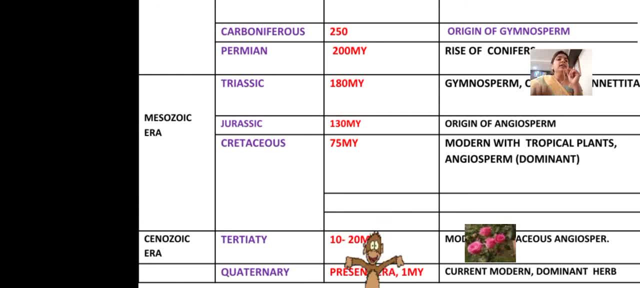 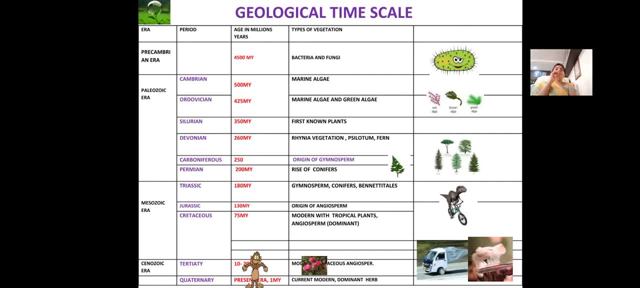 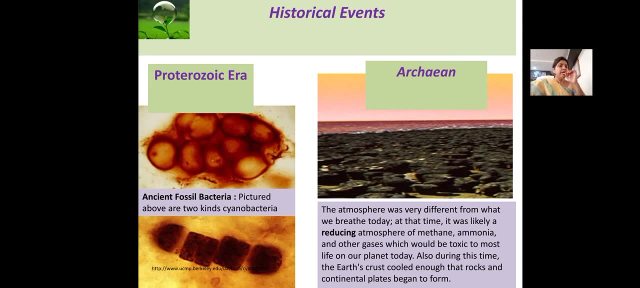 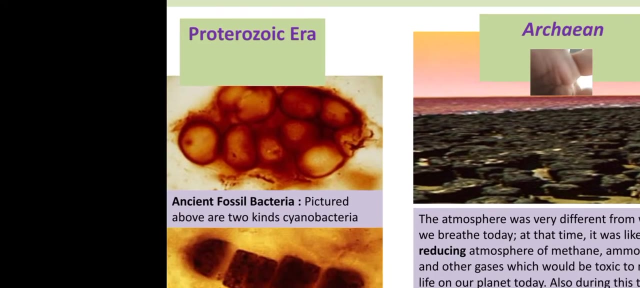 period, mother, okay that it they have to cha geological timescale to me, details today, but he's not okay. up and when, by when, a kick period, but what the next stage? I'm a day honey. he could details, but they upon a high lecture point. I continue. corruptor, a historical events: Midewanda first, protea row, joy Kira. 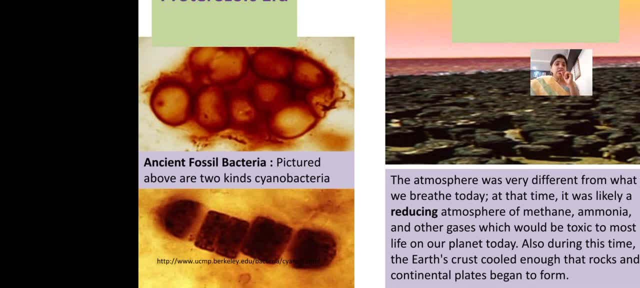 ata. yes, a mother happened. manuscript. or can bacteria jahit and cn? fossil bacteria Gemini, Leia, Nato, Napa, asleep is nothing but the something dug out the earth crushed were called fossil trappella bacteria. chifo signal: Alala headed a picture me, but I'm ordered to hear two kinds of sign of bacteria: hi, J, nitrogen. 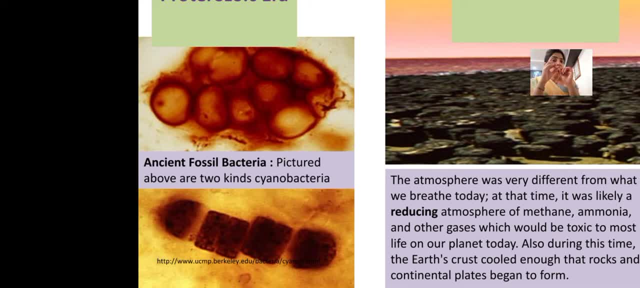 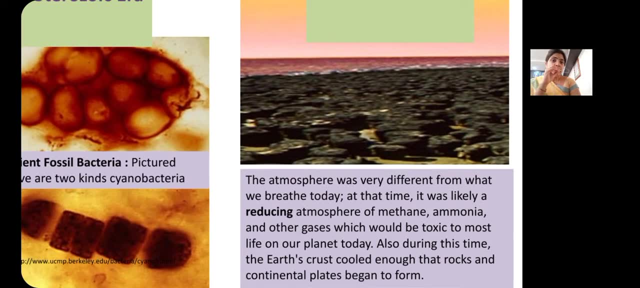 fixation made a couple. motorola answer: okay in nitrogen-fixing bacteria. appellate: Malala head proteolysis. I carry a mother, I'll change the atmosphere. the atmosphere- a bag at it, look as a hotel at. so the atmosphere was very different from what we breathe today at the job. at the banana picture that must be a coupe ago. at that time it. 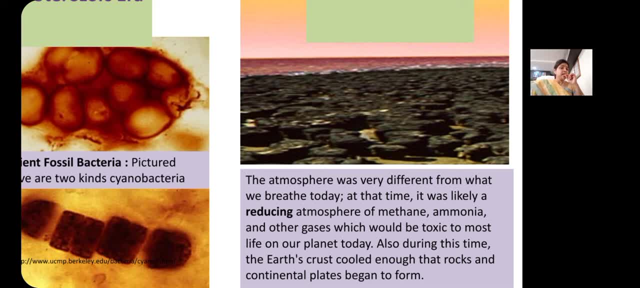 was likely a reducing atmosphere of methane, ammonia and other gases which would be toxic to most life on our plant. today also, during this time, the earth crust cool enough that rocks and continental plates began to form baka. the sata veg veg. a grahan verti man bun bun one top and Mangala verti Chandra. 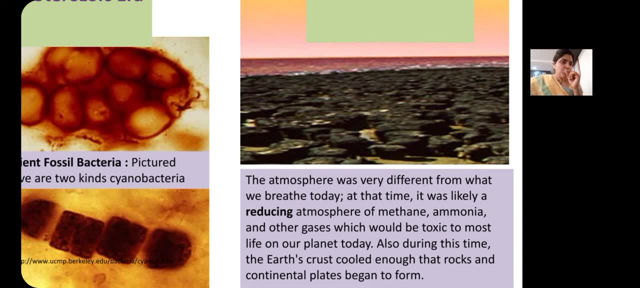 verti J atmosphere at Pune. rocky rocks- I hit it ever put. okay, this is earth saplia atmosphere with a big toxic gases. earth verti with a semi-thin ammonia head- okay, and it could go down as she. earth Houthi, Tila, Purna, cool Vaila. it is 30 millions years, luckily. 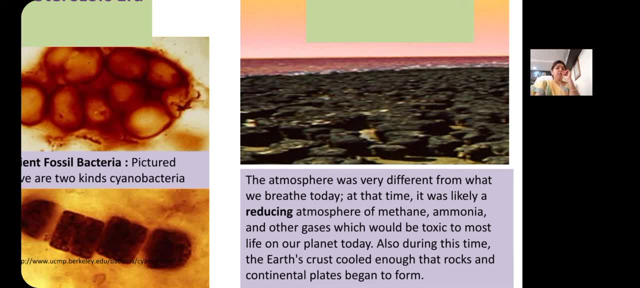 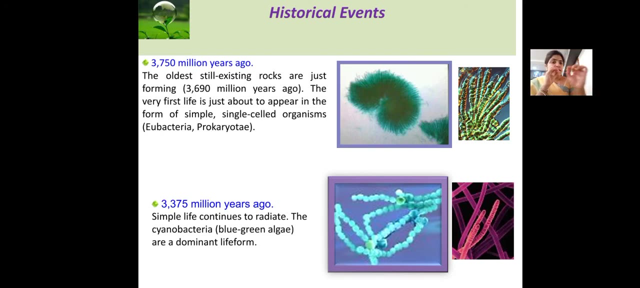 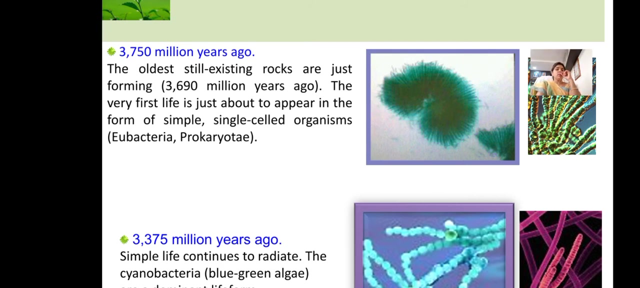 okay, the condition. mother here, bacteria top top tickle, shakali, nitrogen-fixing bacteria, that is the cyanobacteria ticket. and how do? how do a hammock, a horror of a little ugly- they belong, final ugly- take a tenon. third historical events: Madhava heads up Ella 300 and 3,750 millions years ago, the oldest. 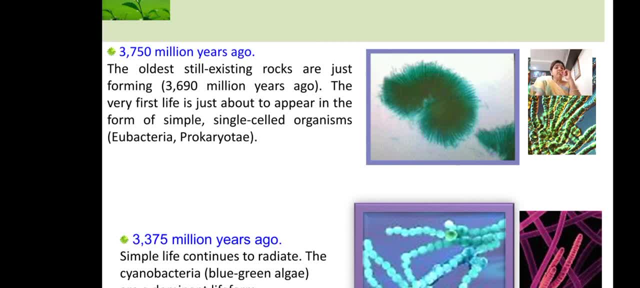 still existing rocks are just forming. the very first life is just about to appear in the form of simple single cell organism called as the you bacteria or prokaryotes mother. the picture delay, let's say you back to your prokaryotes, so they evolves a little at three thousand, three thousand seven and fifty. 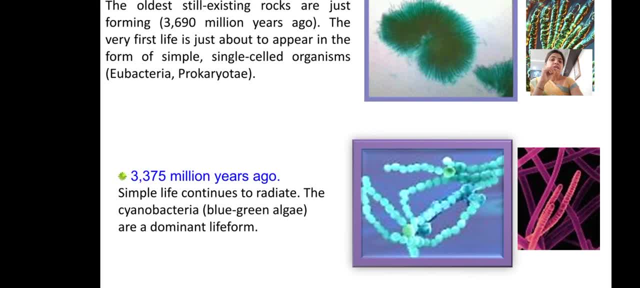 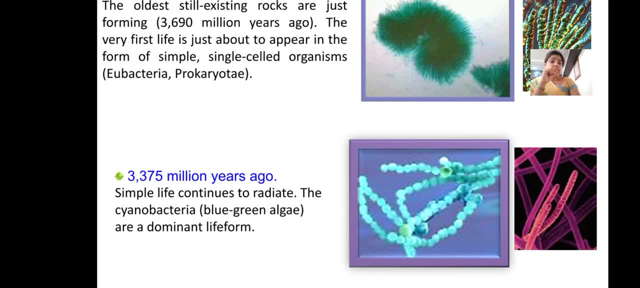 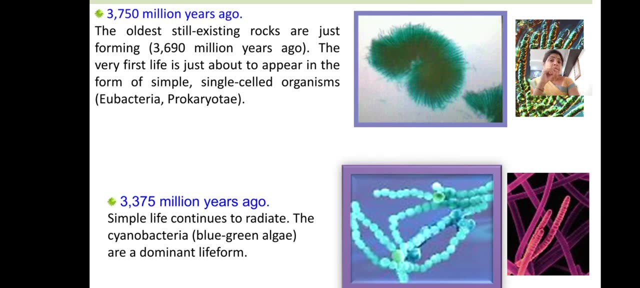 million years ago, then enter three thousand three hundred and seventy five million years ago. simple life continues to radiate. the cyanobacteria blue, green, leaky are the dominant life form, while a kind of a lead single cell organism produce you bacteria. prokaryotes are the earth party and it then enter carat blue. 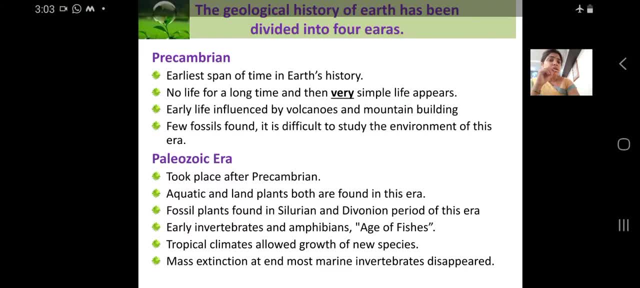 green alky. okay, then enter up and take a key Robbo and a mug. stop guru, pre-cambrian era to him, which I'm a day up and pilots bug it like pre-cambrian Mirama. the car developed a lot. it is the earliest span. 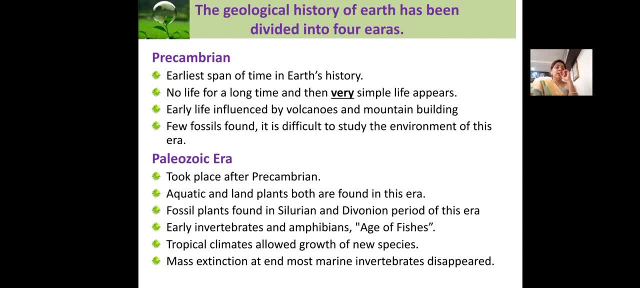 of time in the earth history. no life for a long time and the very simple life appears. sure earth, worthy life is not a mug. J evolves a lot. a very simple form of life appears, Allah. then the early life influenced by volcanoes and mountains, buildings. few fossils found. it is difficult to study the environment of 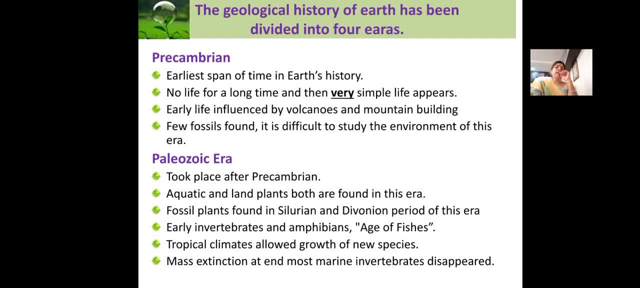 this era, any kind of fossils of the laia, carat, lemur, aliyah. he went our tower Napan, that she environment, she gays, crucial. he kept a moment, Casasin. okay, then enter palliative weck era, sick into narrator: a police regiment. it took place after the 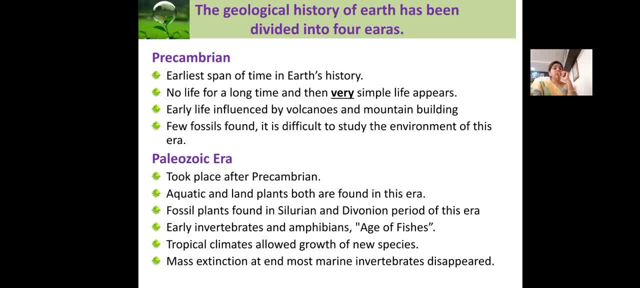 pre-cambrian aquatic and land plans for that pound in this era, TK Alain Paul land tansha hit through be poor phrases. they apply. central area. mother sitc I 거야. mother resindi lelitene as a hero. six pyrrho, luxurious Lillie vaca. 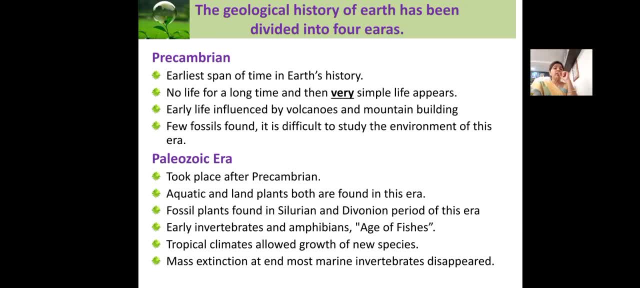 bucket lapper fossil plants found in thisو量. so the D' Benson they had showed before at the Vapi Pippin there are many early in vertical islair and obedience. this is the age of PC, is age of llinha. this is the age of Towsel form like non primary, alors impinary Puckerveen's. this is. 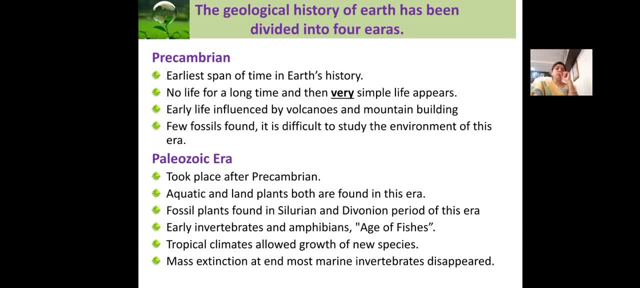 fish, ishman mentality, Allah, tropical climates allowed to grow up new species. mass extinction at the end of marine invertebrate disappear just happen. mental of ki kahi: jay hot a pile a chair. animals give a plans, take as a leap or no, destroys a lecar and then the earth change, Ali and it, they jay pile a chair. 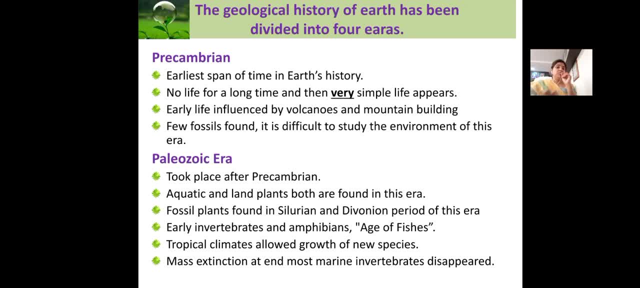 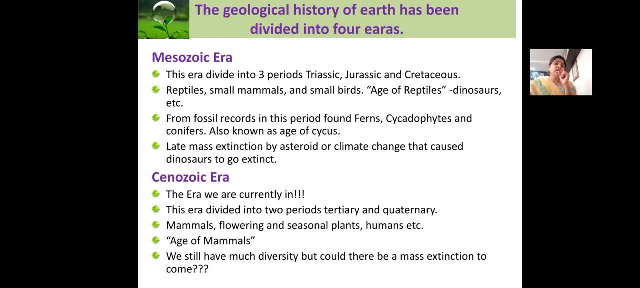 jay animals give a plant set in the environment when they survive in a critical, then under me. so so, Kira, hey, this era divided into three period. that is the triassic Jura- she's Jurassic- and Cretaceous reptiles, small mammals, small birds. this is the age of reptiles, that is, the dinosaurs, etc. okay, from fossil. 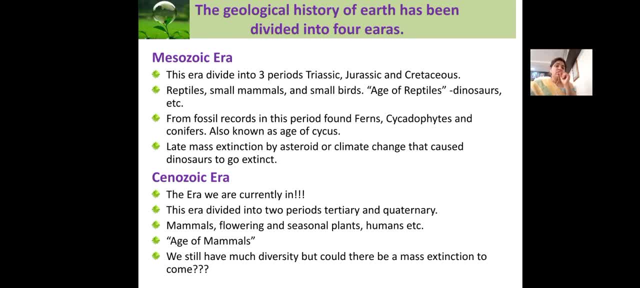 record in this period found ferns and psychedophytes and conifers, also known as the age of cycles. let mass extinction by steroid or climate change that caused dinosaurs to get extinct, go extinct. okay, yeah, era mother panca hot a hoop sorry reptiles with a sir. 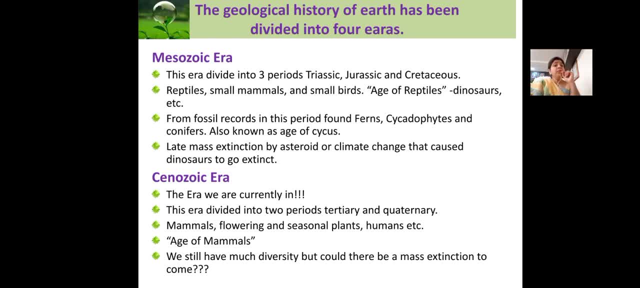 partner. a prani with a this dinosaurs ahead with a tape and guys, a lemme environment change, hello honey the dinosaurs so that it totally casually destroys honey at a pala. a Jalila I, I know it's an inter-op, Cahill, I don't know, catch an inter-op la J modern man say: yeah, yeah, I'm three. 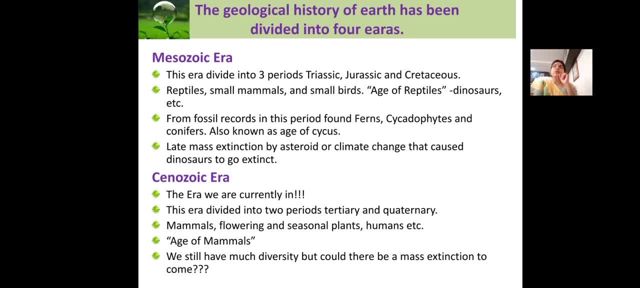 district I. three era's, you shakto, and they come with a animal survival as a kayak hanging. hey, now the Cenozoic era, the Seder. we are currently, in this era, divided into two periods: tertiary, cot and Quaternary. mammals, flowering and seasonal plant, humans, etc. found in this era. this is the 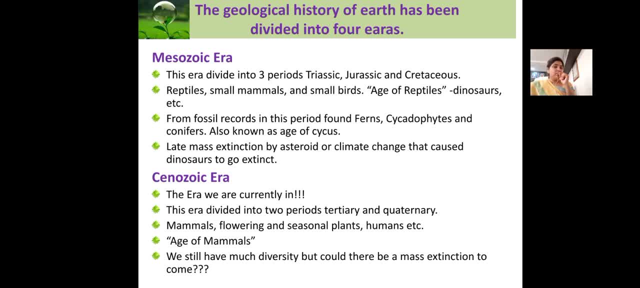 age of mammals. okay, we still have much diversity, but could there be a mass extension to come, he upon happen era totally destroyed own? yeah, that's my lucky. after mammals could love a general, hey, we all don't know. okay, okay, it's a apply her geological time scale. so a topic with a model, first one, a complete. 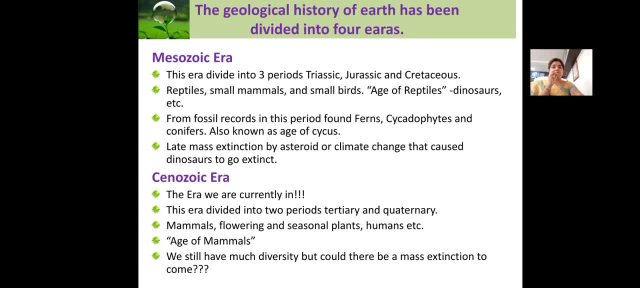 Salela. hey, next lecture, mother happened. detail procedure: bagu fossilization G. okay, mr of, get there. 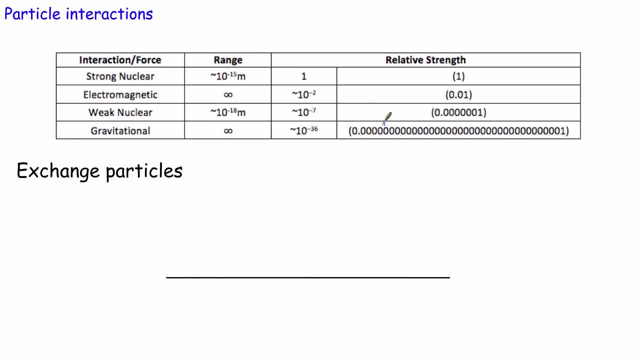 Hello and welcome to this video where today we're going to be looking at how particles actually interact with each other. Now, there are four different types of interaction altogether. On an everyday scale, we see lots and lots of different interactions or lots and lots of different forces. So we see things like weight, we see things like air resistance. 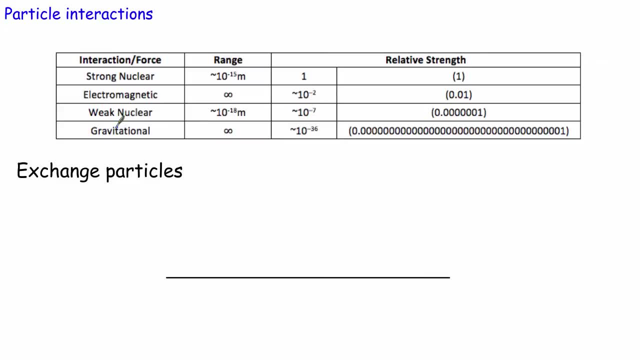 and friction, lots and lots of different types of forces, But really they just boil down to four different forces or four different interactions. Two of these we know really really well. Obviously, we know the gravitational force. we experience it all the time. Now, 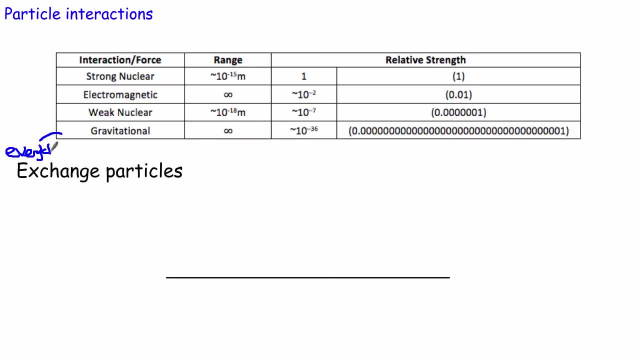 every single thing feels this gravitational interaction or gravitational force. You're feeling it now. it's the attraction between you and the earth, it's the thing that keeps you on the floor, basically. But every single thing in the universe feels some sort of gravitational. 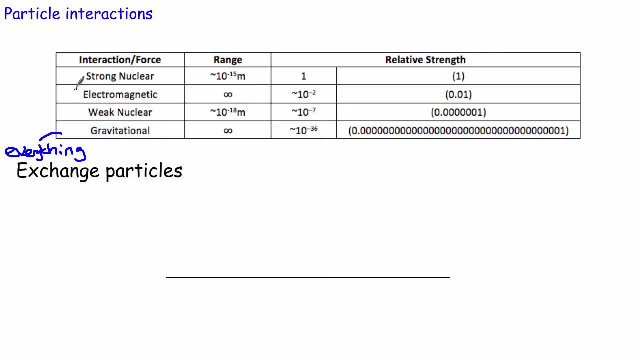 attraction, So this interaction works with any particles whatsoever. We also know quite a lot about this electromagnetic interaction. We've been using this for quite a long time. we use this at GCSE because anything that's charged, so anything that either has a positive or a negative charge, feels this electromagnetic interaction. If 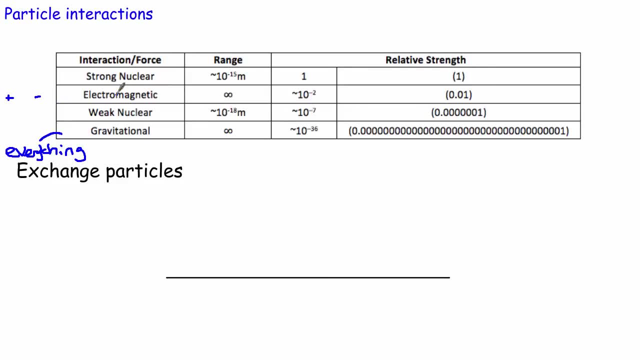 you're a neutral particle, like a neutron for example, you don't feel this electromagnetic interaction. So you only feel it if you're a charged particle And obviously, if you've got something that's positive, something that's negative, then the interaction you feel is: